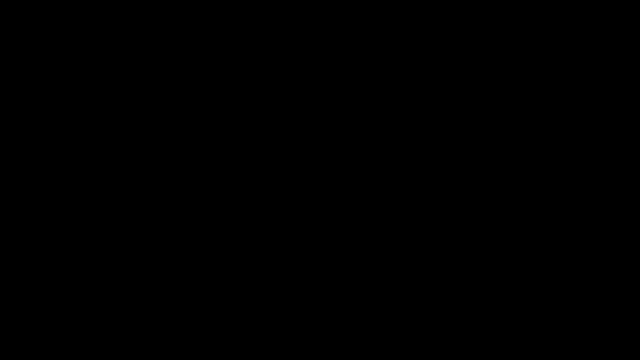 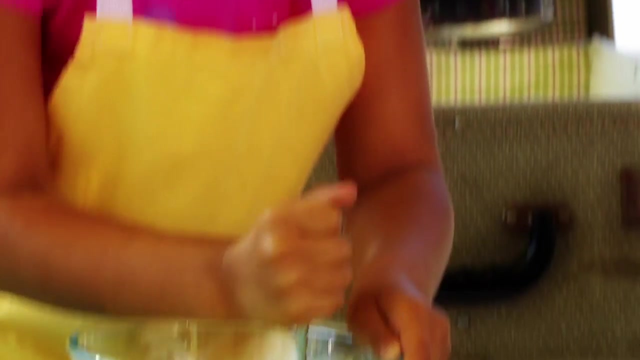 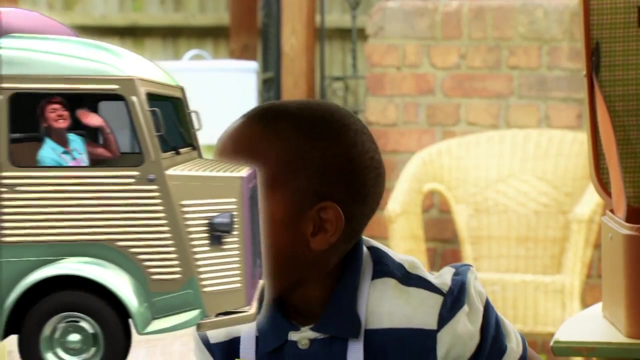 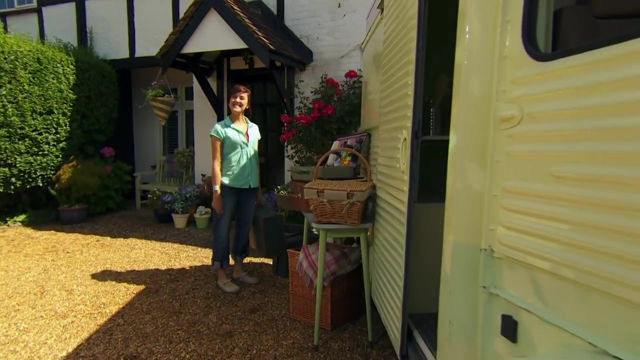 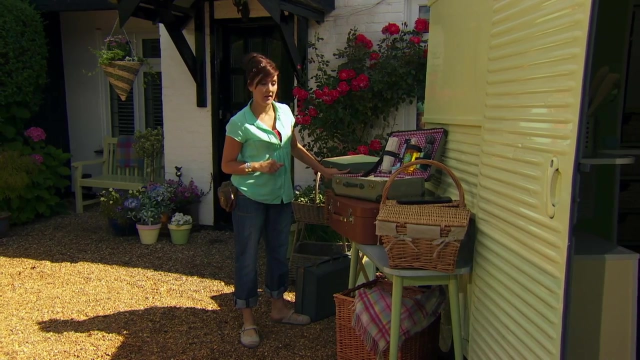 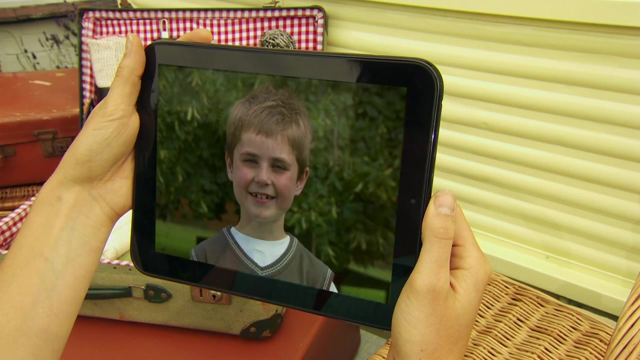 With you. Hello, Oh, great to see you. I'm just getting everything ready to go on a journey and I hope that you're going to come with me and make some new friends. Aha, Hi, Katie, I love bike rides and my favourite fruit is blackcurrants. Oh, that's exciting, Katie. 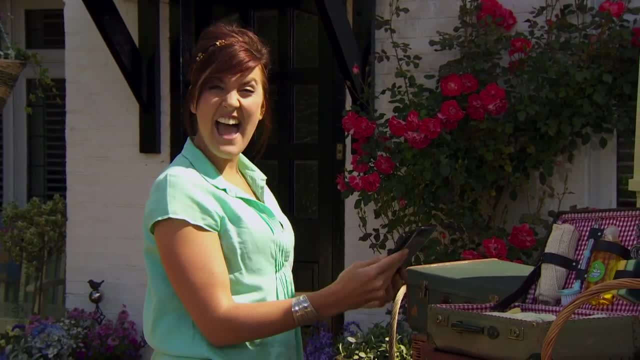 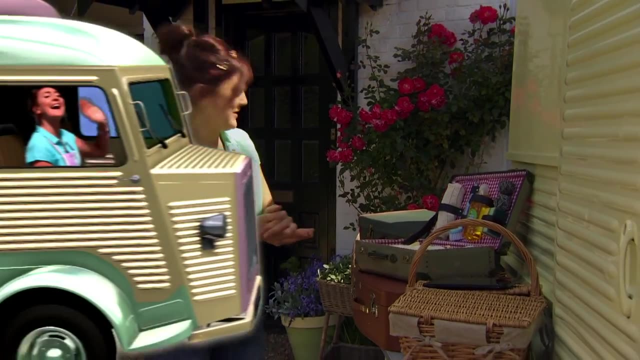 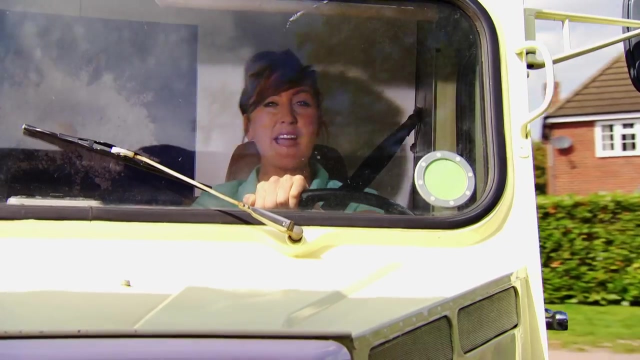 can you cook with me please? I certainly can, Sam, and I love cycling on my bike, and you can cook with me too, So let's pack up and go. I've been on a journey and I'm coming to you. It's going to be busy and there's lots to do. Get ready to help, join in, and 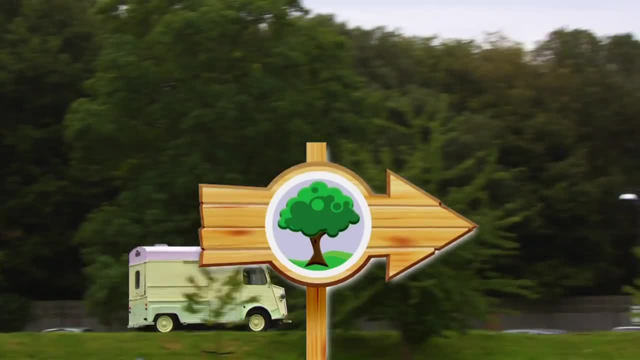 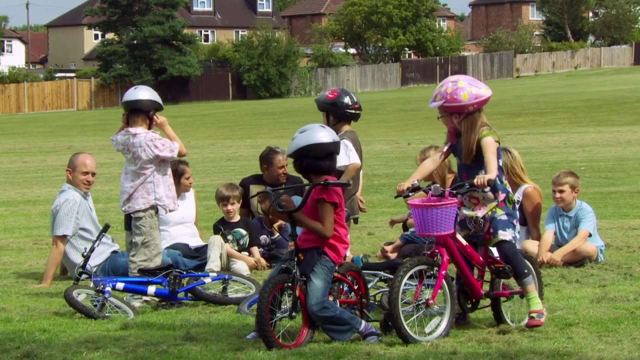 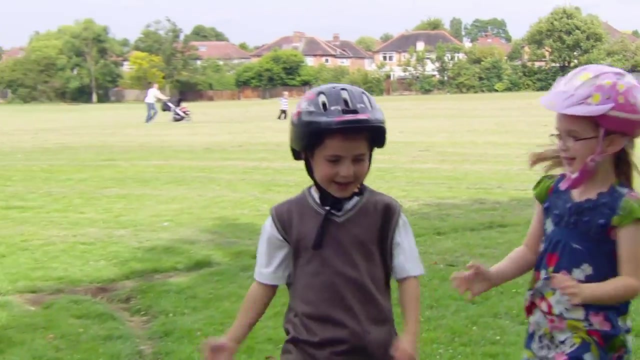 have fun. Let's cook a feast for everyone. Here we are at the park where I've been invited by Sam, And there he is, over there with all his friends. Hi, everyone, Hi, Come on over. Oh, it's great to see you all. So, Sam, are these all your friends? Yes, What are your? 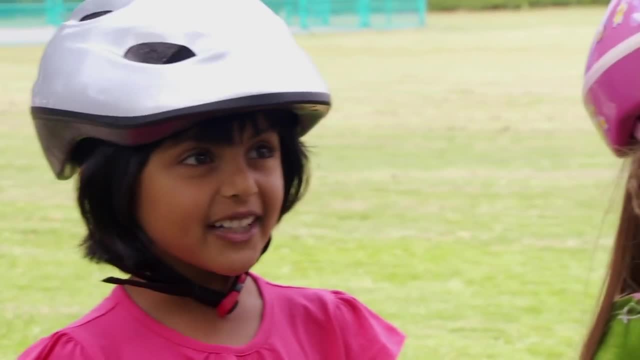 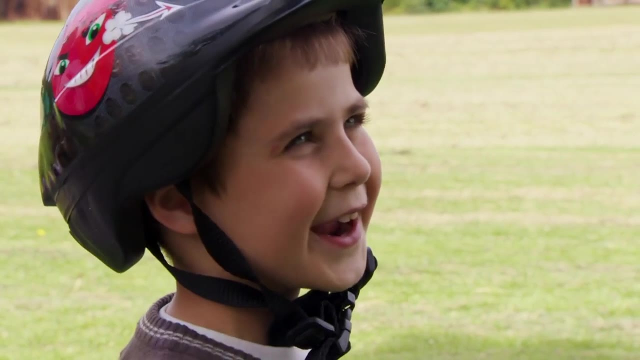 names: Eddie, Megan, Ria. Oh, it's great to meet you all. Hey, Sam, what are we going to do today? Make some food for our bike ride. I have got such a delicious recipe to make with you all. Why. 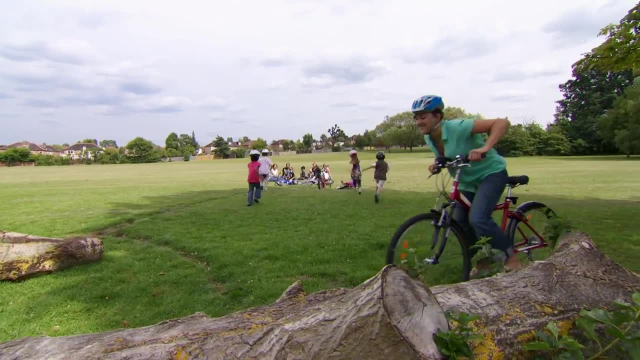 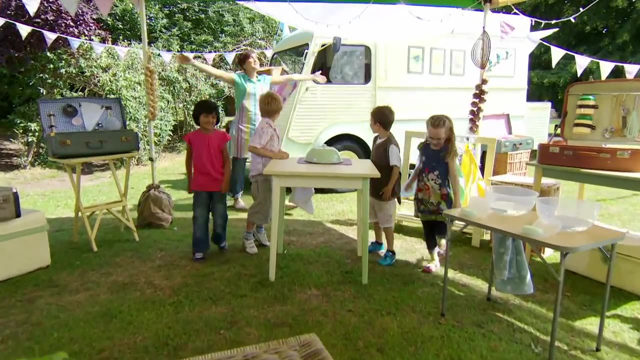 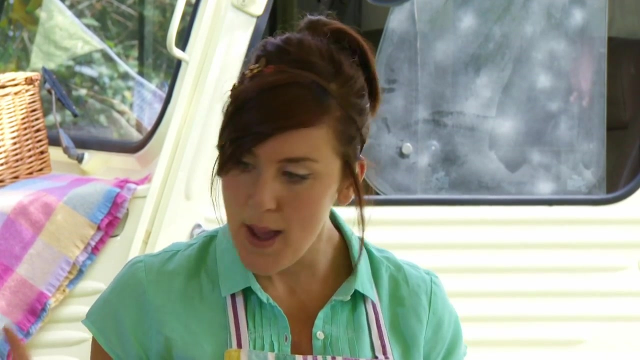 don't you get your bikes and I'll show you what it is? Yay, Welcome to my outdoor kitchen. Hey, do you want to know what we're going to cook today? Yeah, Okay, today's recipe is baked rice- Blackcurrant rice. 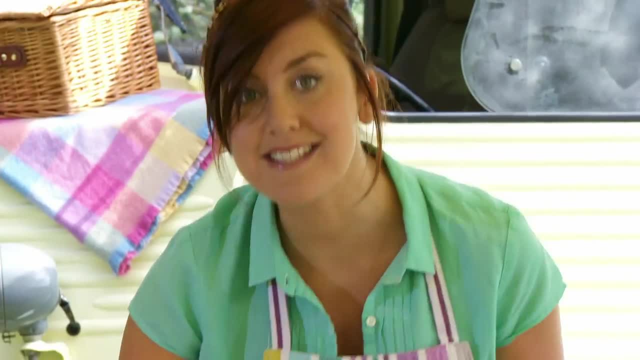 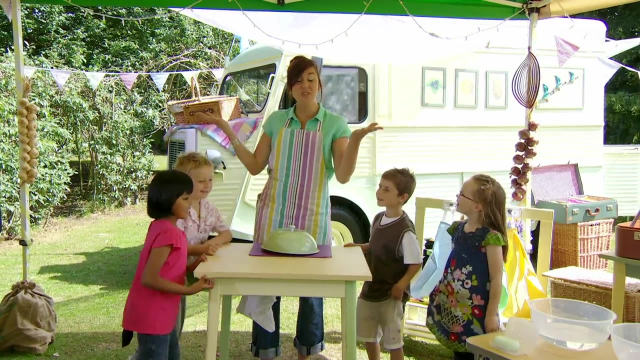 Before we get started on the cooking, there's something really important that we've got to do first. Does anyone know what it is? Wash our hands. You've got it. We've got to wash our hands, of course, So let's get going. 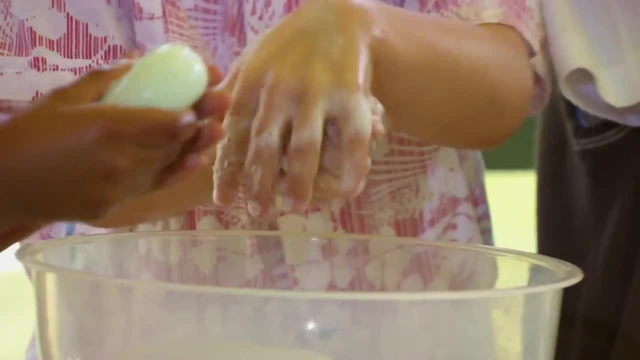 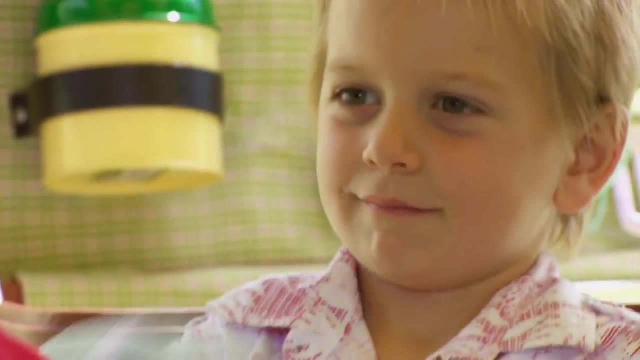 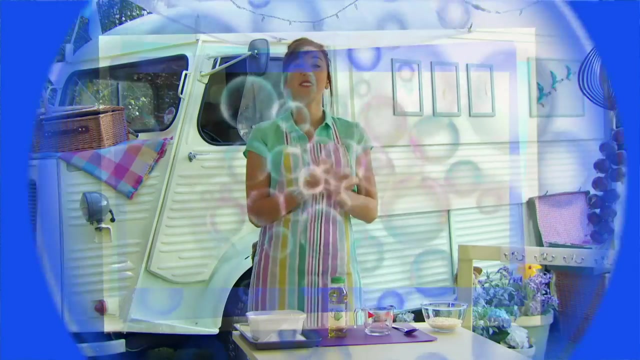 Roll up your sleeves, Give your hands a wash with slippy dippy soap: Splish, splash, blosh. Wash your hands, Wash and dry. Sleeves rolled up, Apron tied: What can you do? I can cook. 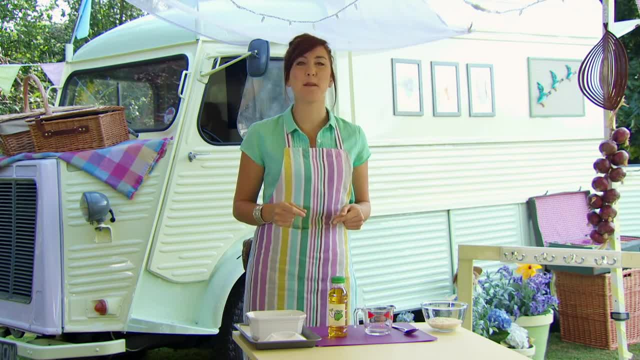 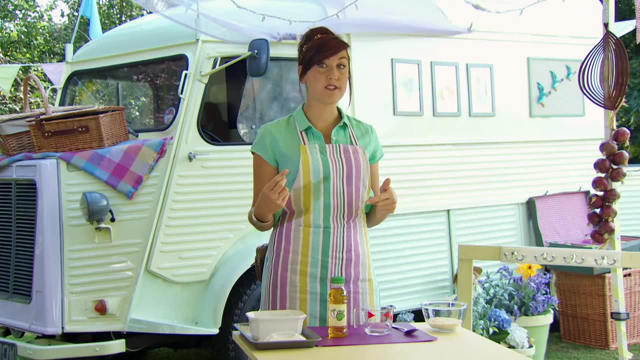 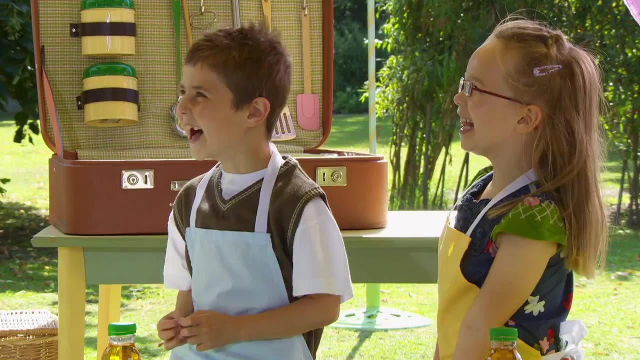 Let's get started Now. the first thing we need for our baked blackcurrant rice is apple juice. How do you normally get juice out of fruit? You squeeze it Like this. you mean Squeeze? Yeah, Well, go on then. Why don't you squeeze with me? You can join in too Ready. 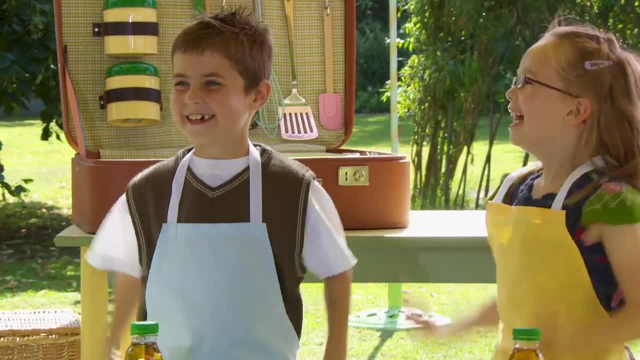 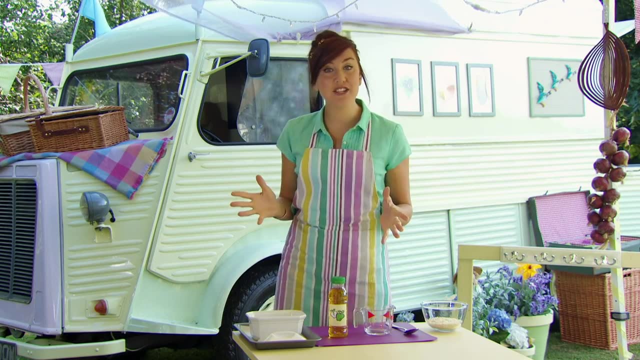 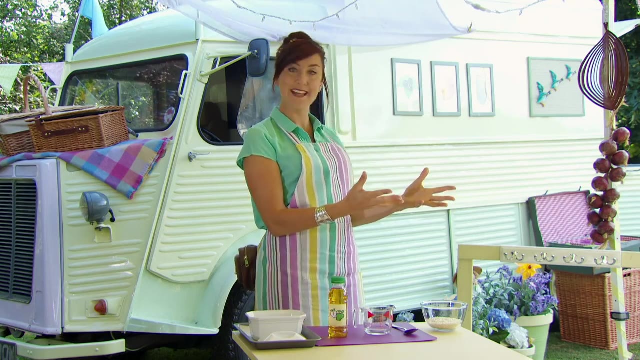 Squeeze, And when you've done that, you get lovely juice, just like this apple juice that we've got here in a bottle. So we need to measure it, And to do that we need to work in pairs. One person's going to be the pourer and the other person is going to be the watcher. Now 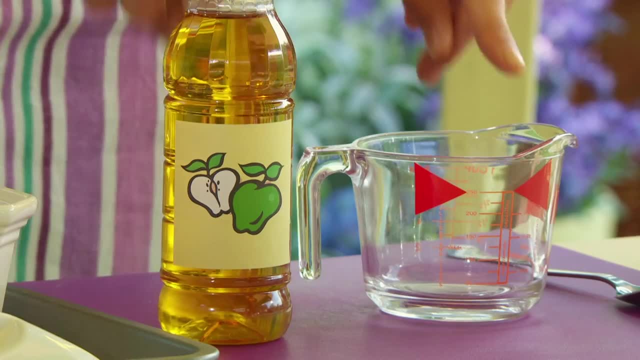 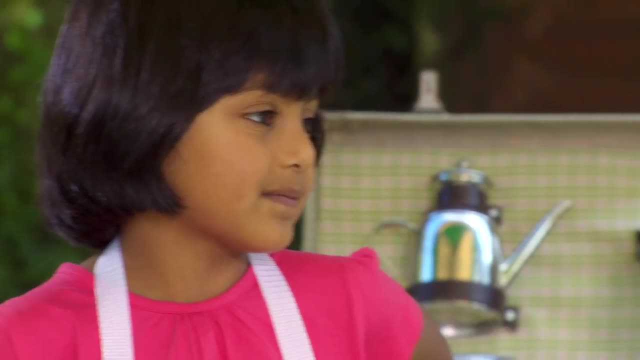 the pourer needs to pour the apple juice into this jug that we've got on our mats. We're going to put it on our mats And the watcher needs to make sure that the pourer fills the jug up to where the red arrows are pointing. Can you see that line, everyone? 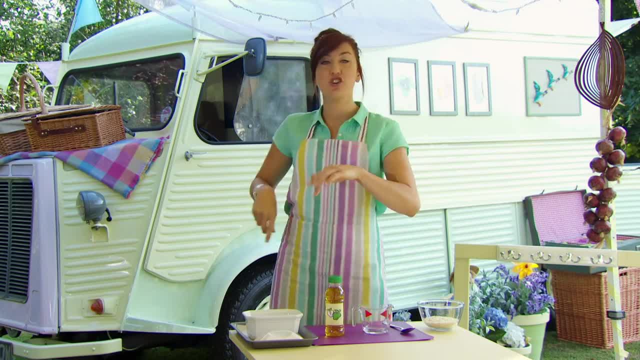 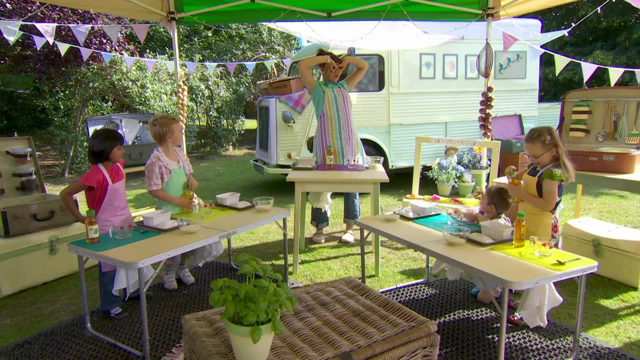 Yeah, Yeah, OK, that's really important, And to be the watcher, you need to put on your watching goggles like this. You got your watching goggles, Yeah Well, let's have a look. then Can you be a watcher as well? Brilliant, So, everybody. 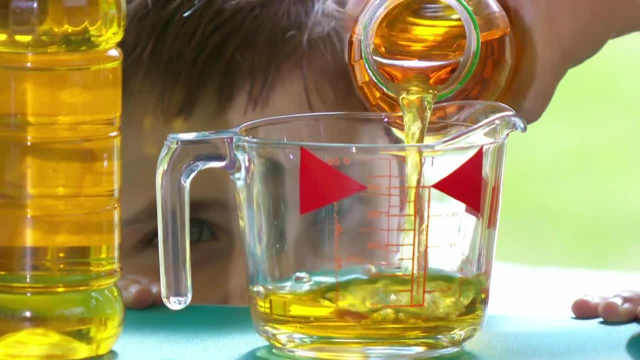 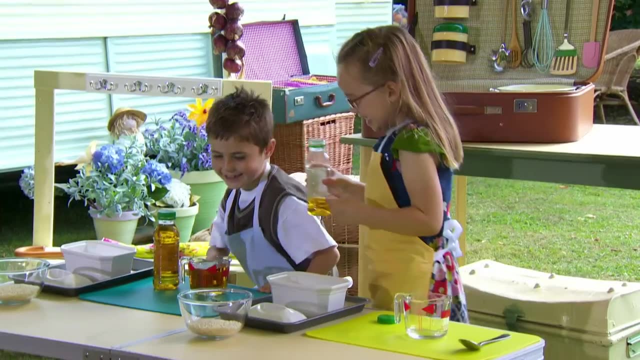 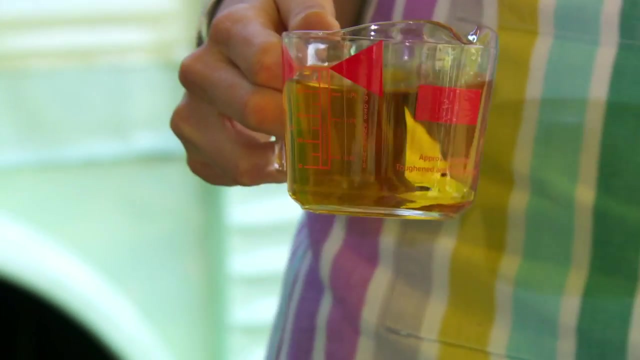 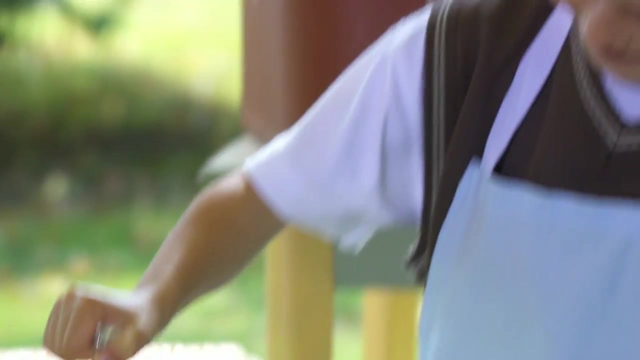 let's get pouring Off. you go Watch carefully. OK, Tell her when to stop, Sam, Stop. Did you do it Brilliant? Take your jug of apple juice and pour it into your dish- One, two, three splash. 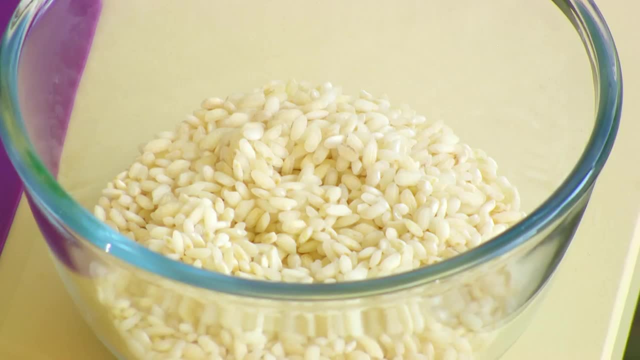 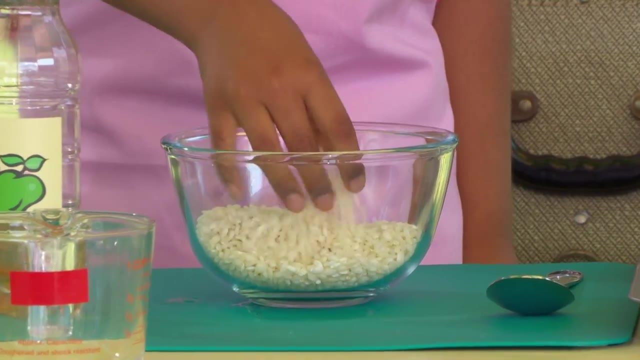 The next thing we need is some arborio rice, And this rice is great to use for risottos and rice puddings. Does it feel nice? Yeah, Yeah, Yeah, Ooh, it feels all funny on my fingers. Yeah, me too. 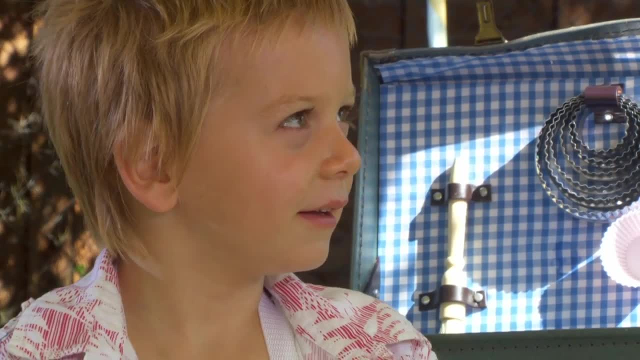 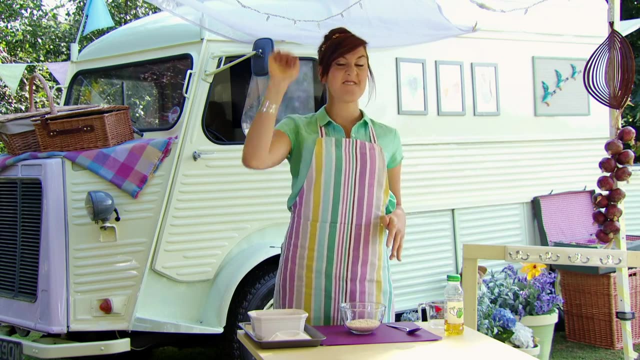 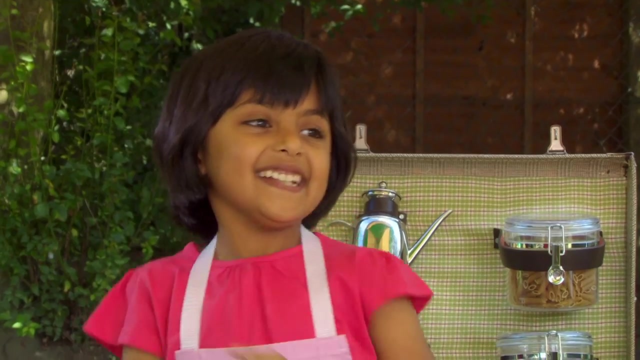 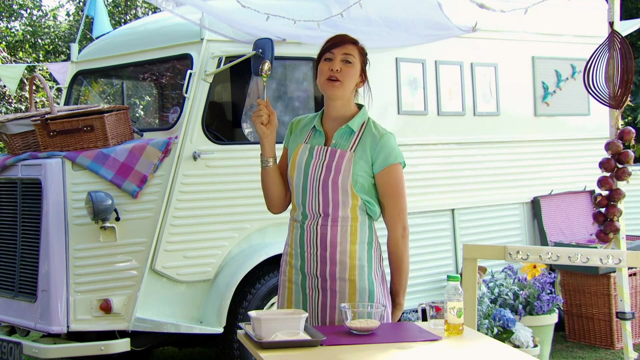 What sound does it make? Rain? Let's listen. Oh yes, It does sound like rain. Now we need to measure five dessert spoonfuls of arborio rice. How many dessert spoonfuls? Five, That's it. And to do that, we need to use our good friend, Mr Spoon. Hello, Mr Spoon. 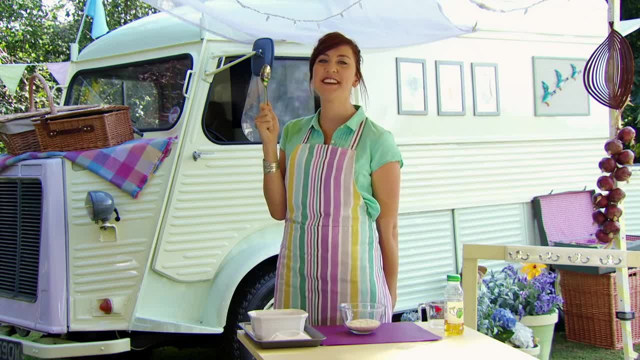 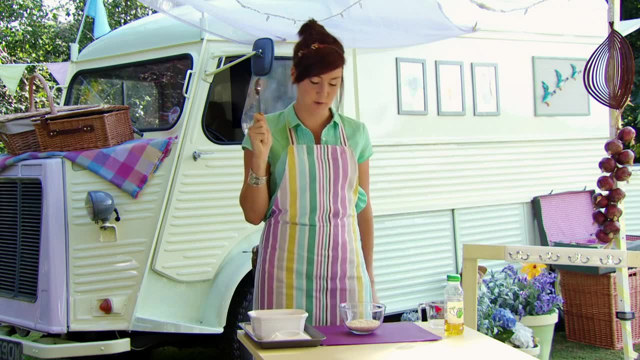 Hello, Oh hello, Katie. How are you today? I'm very well, thanks. How are you? Oh, fantastic, Can't wait to do some measuring. OK, Mr Spoon, Let's measure five dessert spoonfuls of our arborio rice. Ready, Here's. 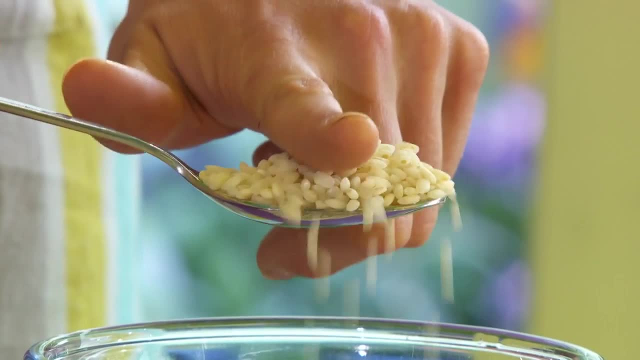 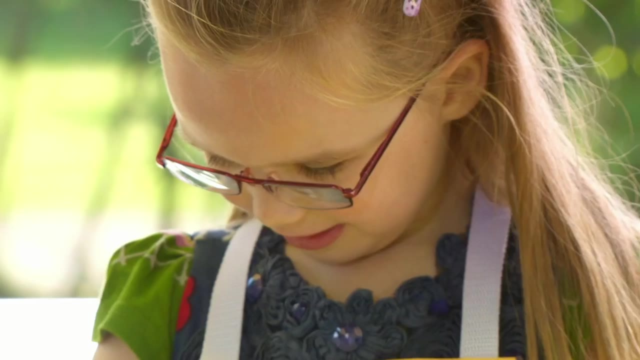 one And pat it. so it's nice and flat: Pat, pat, pat, pat, pat, And then put it into your dish with the apple juice, And when you've done your fifth one, you just put your spoon back into your bowl. 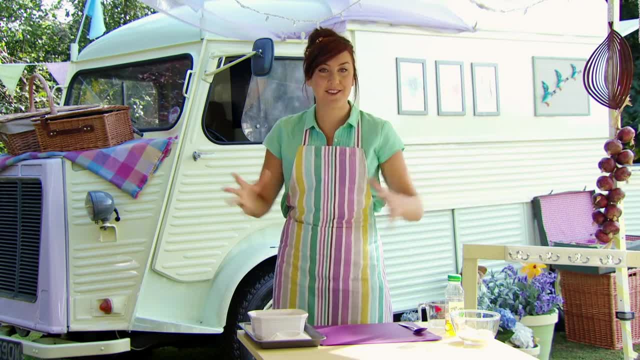 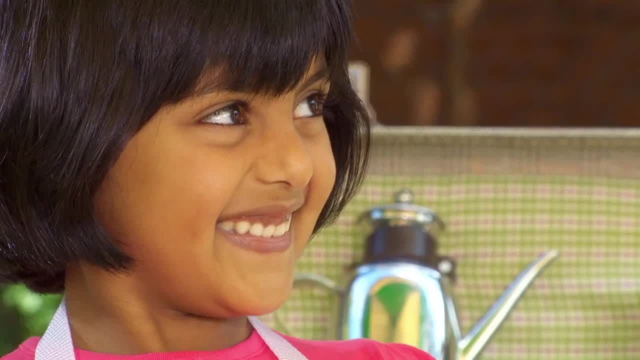 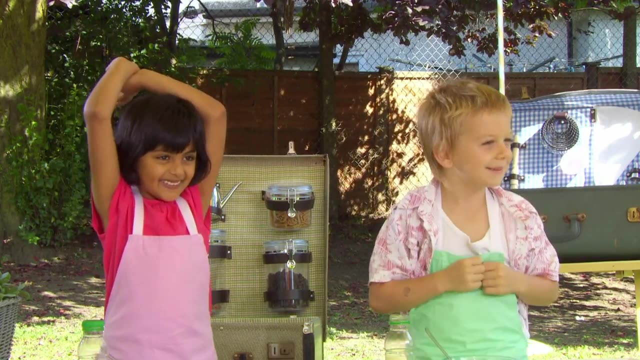 Now what's going to happen is quite exciting. The rice is going to soak up all of the apple juice like this. Should we all pretend to soak up the apple juice altogether? You can join in with us: Ready, Brilliant. So what do you think we're going to need next in this recipe? What's next? 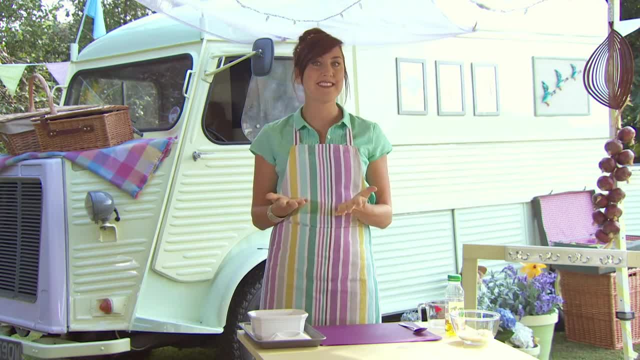 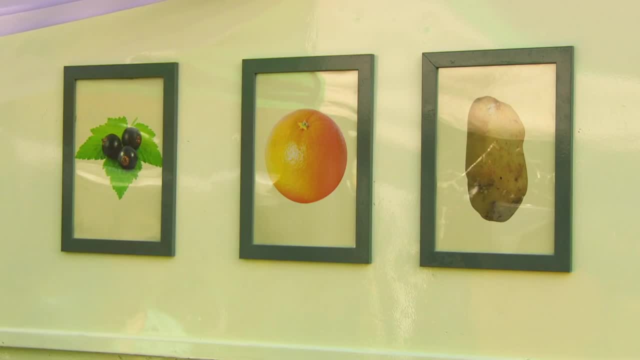 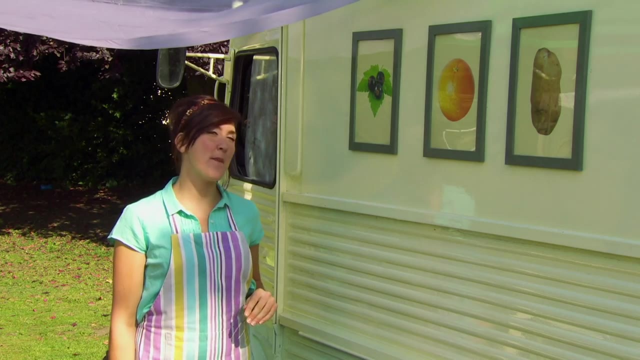 Well, let us see if you can guess what it could be. So we have got a potato, an orange and some blackcurrants. What would you choose for our baked blackcurrant rice? Oh, I know, I'll give you some clues. The special ingredient. 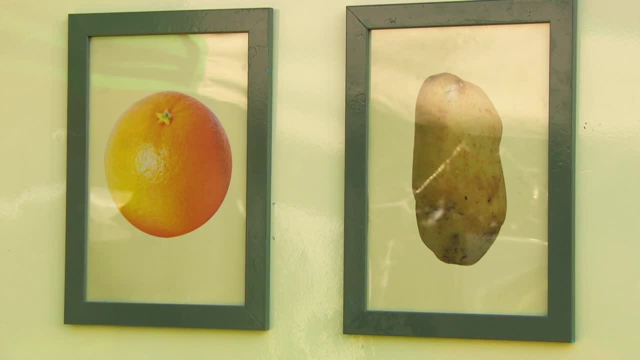 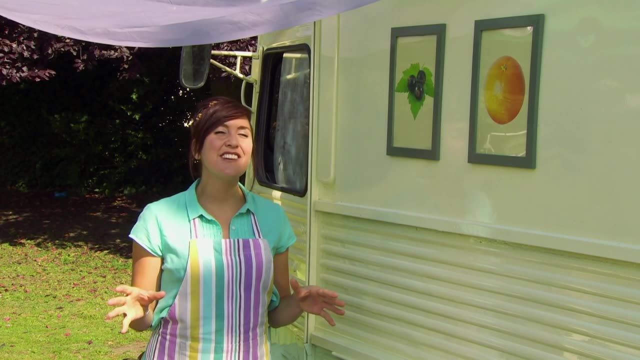 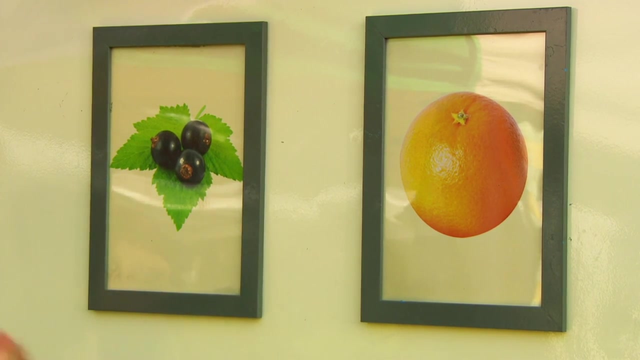 is a fruit. Well, potatoes are a vegetable, aren't they? So we can take that one away. There we go. OK, I'll give you another clue. The special ingredient is a fruit that goes on the bushes. Well, oranges grow on trees, don't they? So we can take that one away. 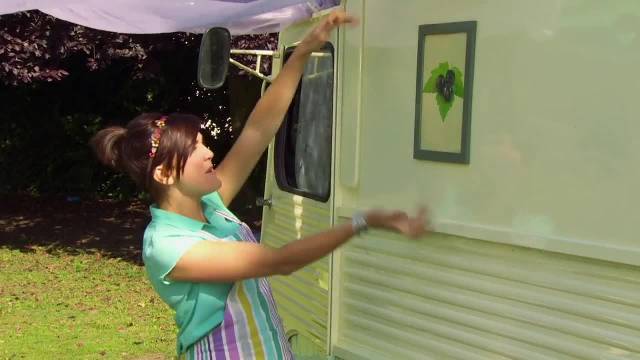 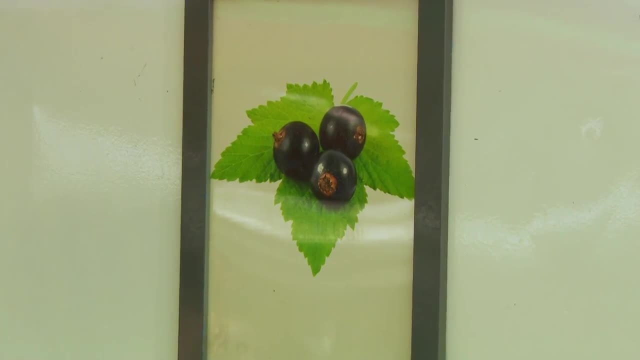 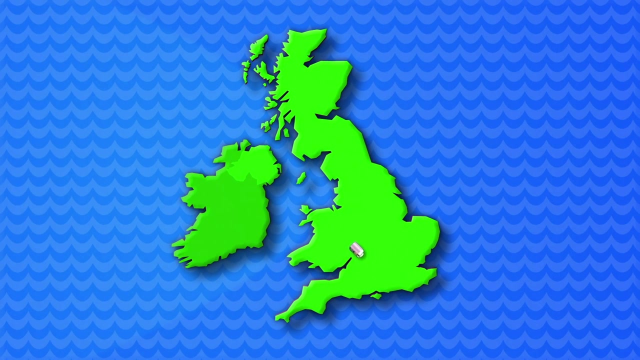 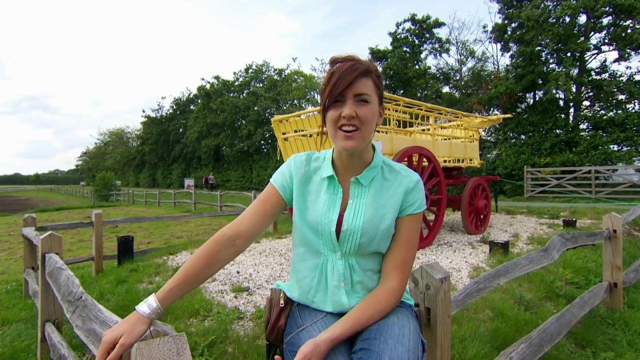 too, Which leaves us with blackcurrants. We're going to need some blackcurrants for our baked blackcurrant rice, And earlier on I went to find some. I've come to Isha in Surrey where I'm going to try and find some blackcurrants, And I've 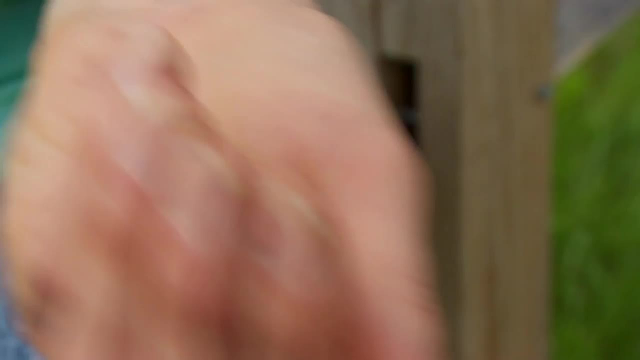 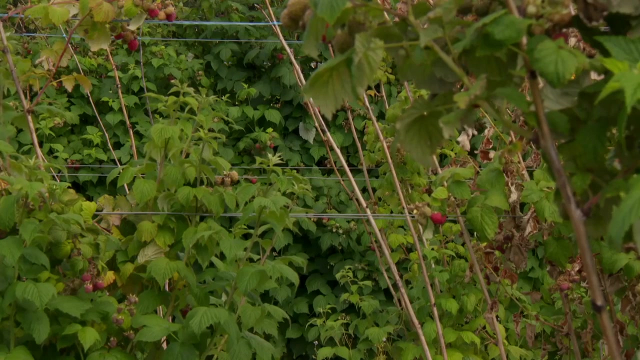 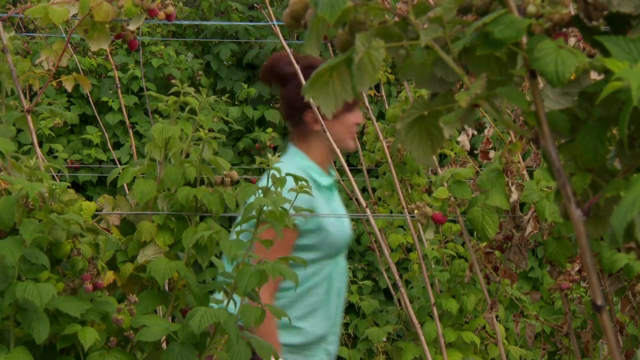 come to a farm where you can pick your own. Now, these are what we're looking for, And they're quite small, aren't they? Should we go and find some? Come on, Wow, that's a lot of blackcurrants. 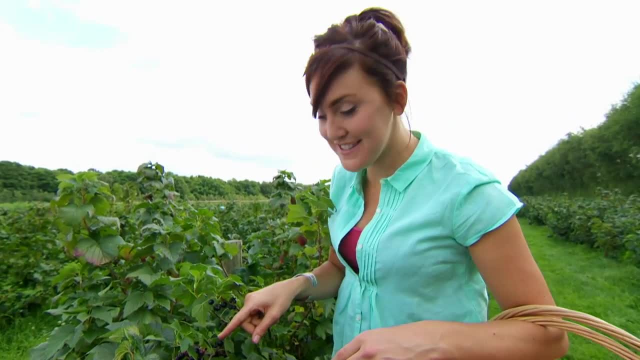 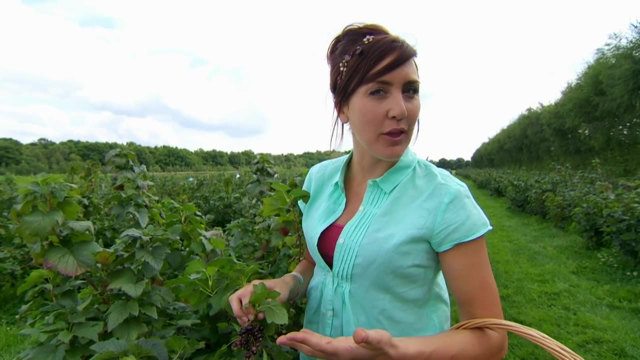 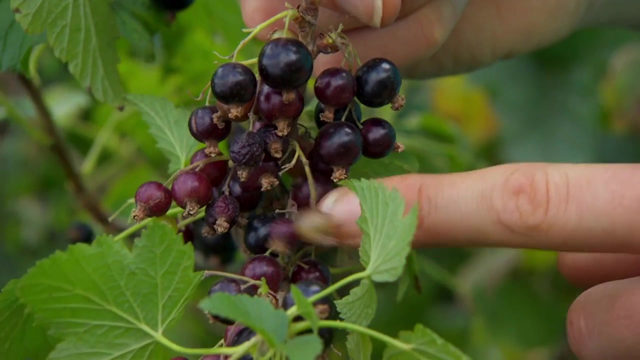 Wow, look how many blackcurrants there are, And you can see that they all grow in a bunch. But you have to be really careful when you're picking them, because you don't want to squash them. The darker ones are perfect for us to pick, But the red ones aren't quite ripe yet. 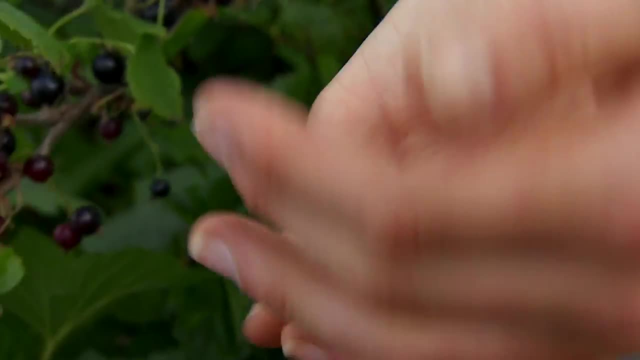 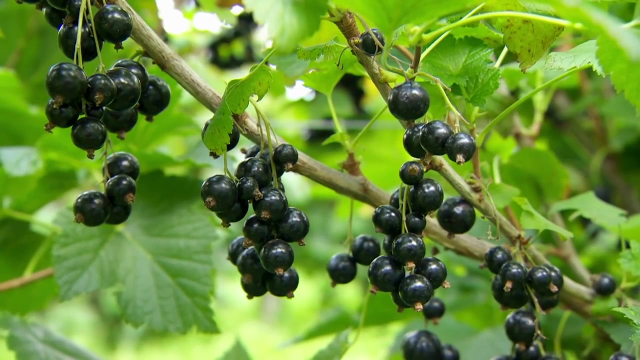 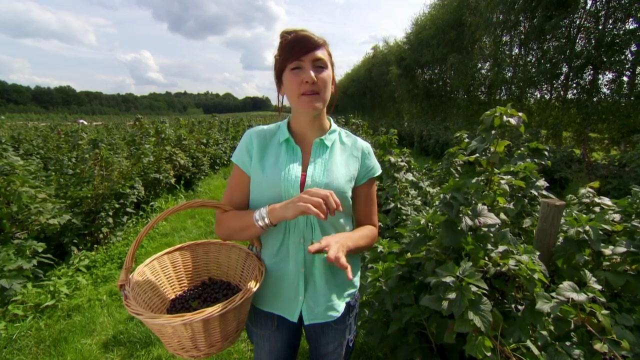 so we won't pick those ones. This is great fun. There are hundreds of them. There we go. I think that's enough blackcurrants for everyone, And now I just need to give these a wash and then they'll be ready to use in our baked blackcurrant rice. 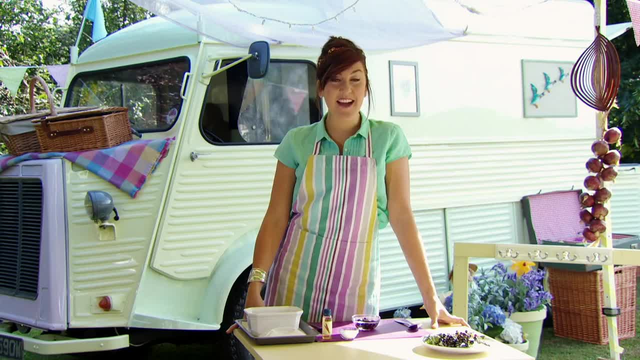 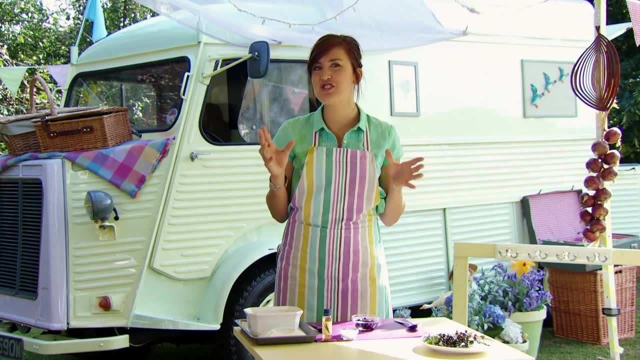 I loved picking all those blackcurrants and I couldn't believe how many there were. But I've got a question for you. What colour do you think blackcurrant juice is? Purple, Purple, Purple. Why don't we squash one and let's have a look? 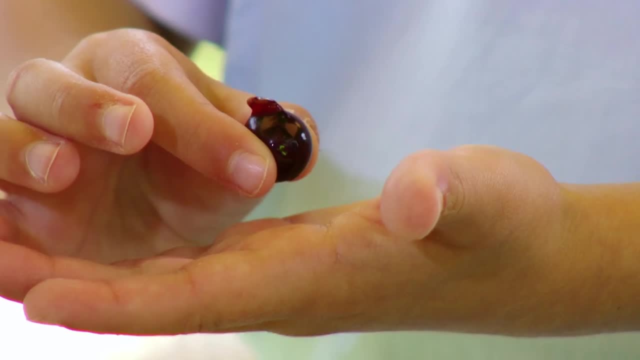 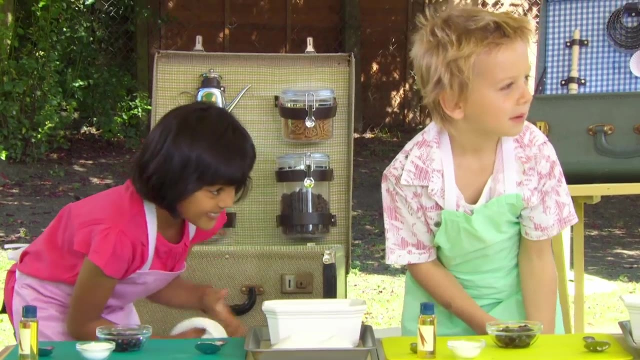 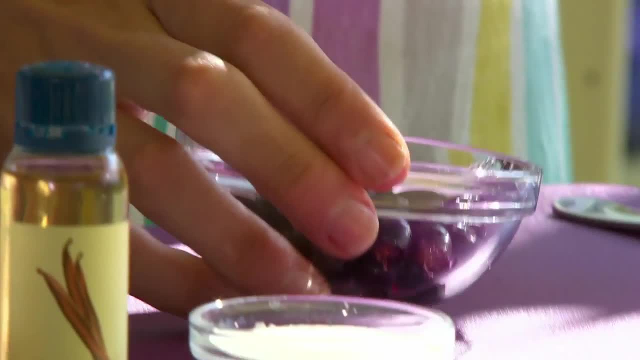 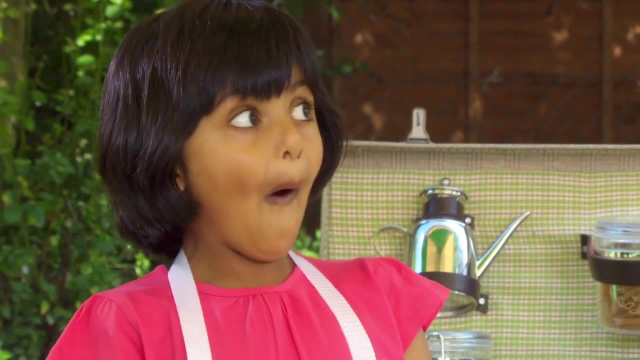 Now we need to add these blackcurrants into our dish, So let's sprinkle them in When the blackcurrants go in the oven. they're going to pop because it gets so hot in the oven. they go like this Pop. 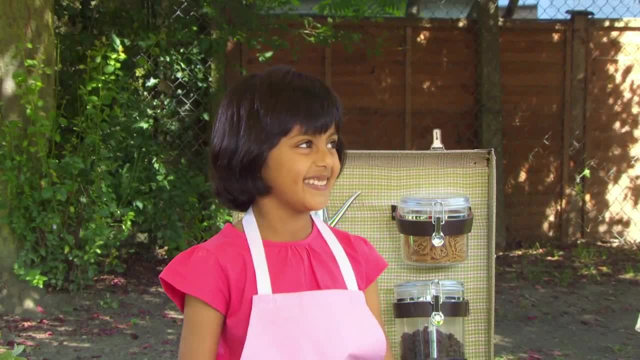 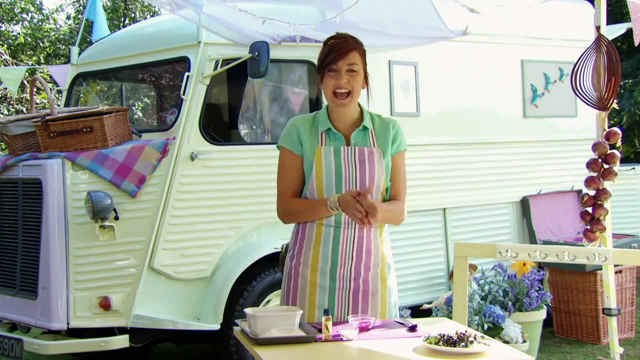 Can you do that? Yeah, Pop Pop, And this time you can join in with the popping. One, two, three Pop Pop. OK, now the next thing we need to add is some sugar, and we're going to use caster sugar. 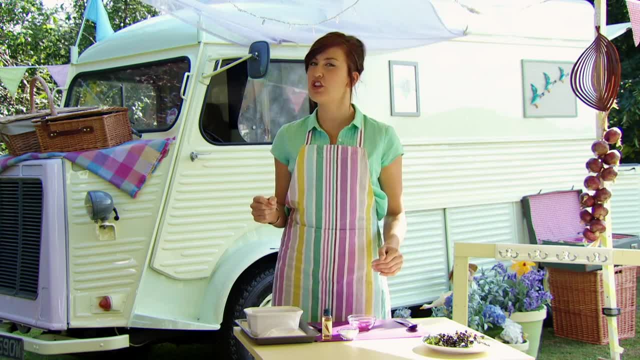 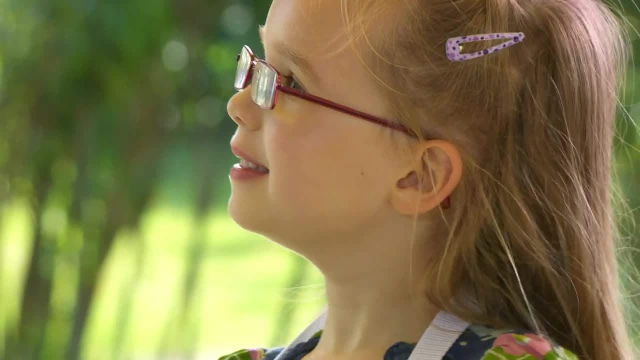 Now, caster sugar's a little bit different to the kind of sugar that you might be used to using when you're at home, and that's because the granules, which are the little pieces, are much smaller. Now we need to sprinkle this sugar into our dish and we're going. 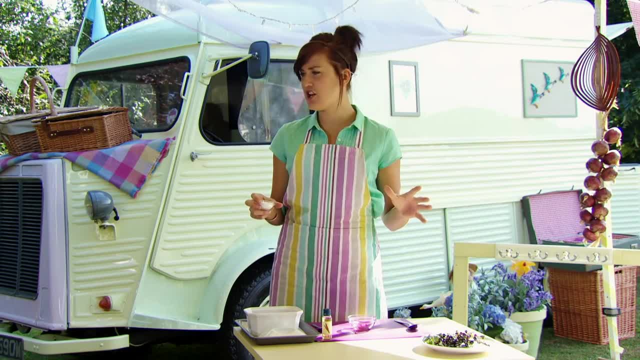 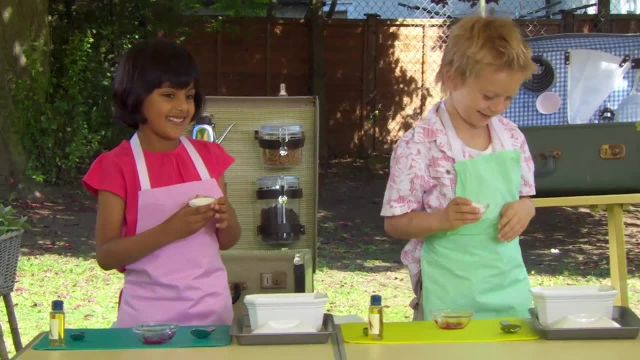 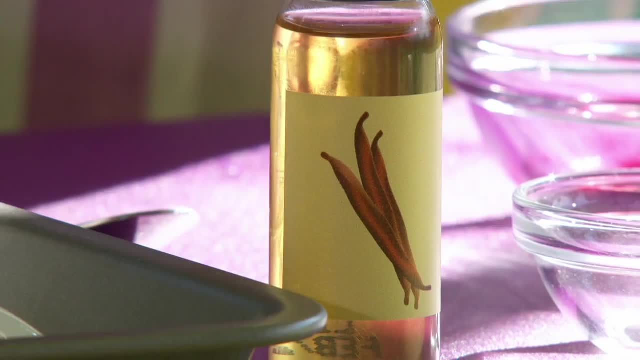 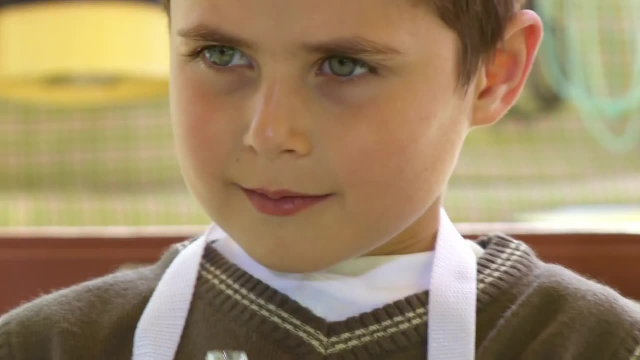 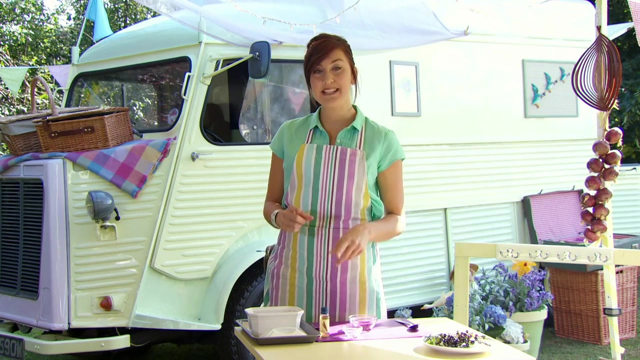 That's a good sugar shuffle, Eddie. Now the next thing we're going to add is vanilla extract. Should we give it a smell before we add it? Yeah, OK, Eddie. what does it smell? like Ice cream, Vanilla ice cream. Do you like vanilla ice cream? I love it, And we need to measure half. 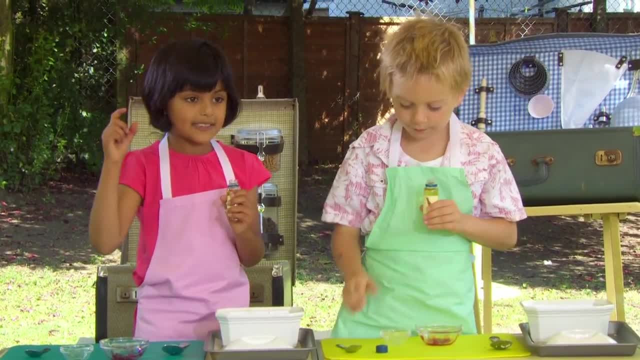 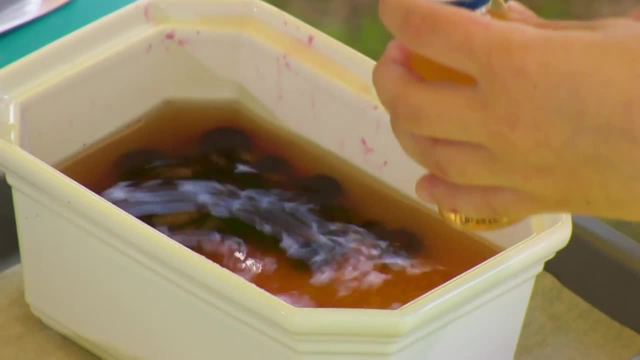 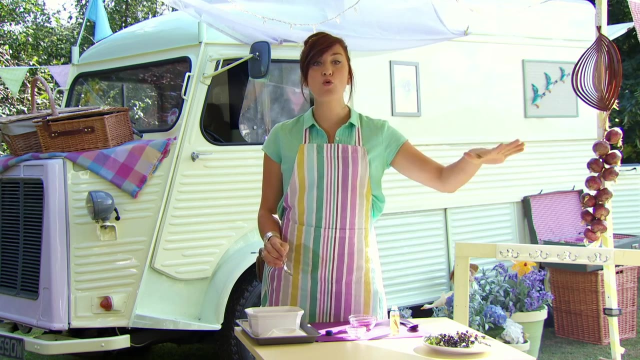 a teaspoon of vanilla extract. So hold your teaspoon over your dish and, very carefully, That's enough- and splash it in. Now the last thing we're going to do is give everything in our dish a good stir, But we have to give it a really slow stir, because otherwise all the things are going to splash. 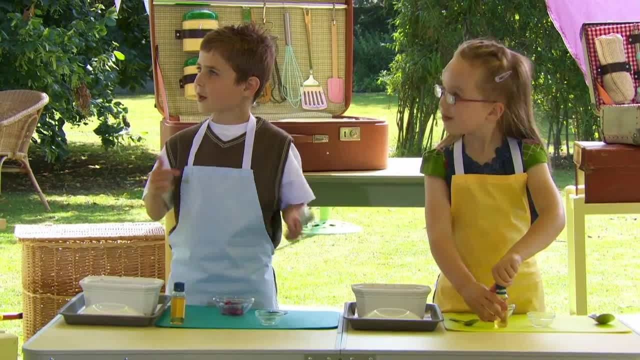 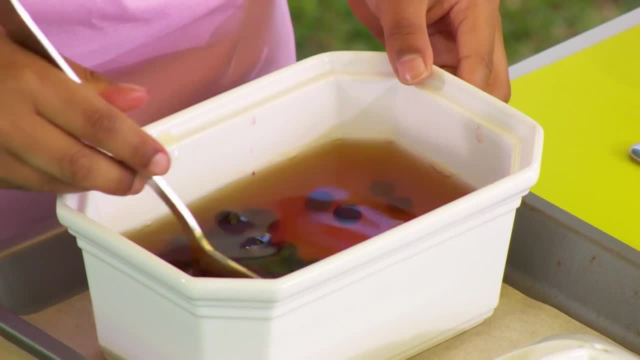 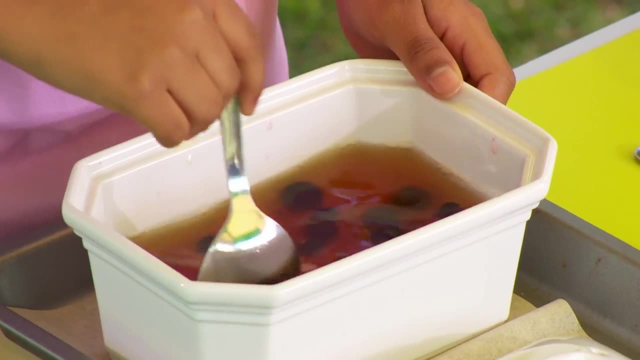 beep, Have you done the slow button And give it a nice slow stir? Ooh, the colour's coming out of the black currants in mine, Yeah, I can see the juices coming out because it's red all around. Is that the juice from the black currants? 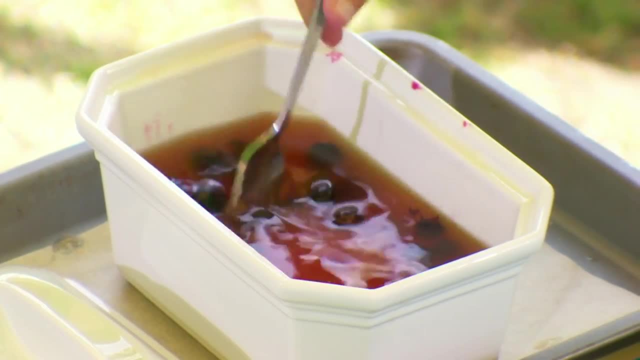 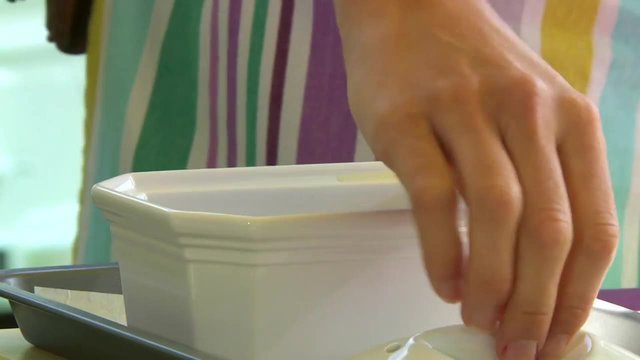 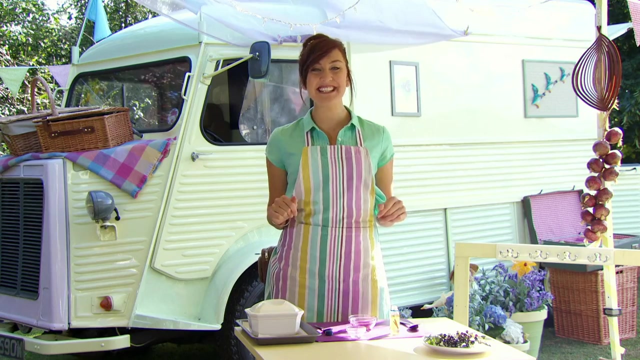 Yeah, What do you think is happening to the sugar? It's gone. Do you think it's dissolved like this? Yeah, OK, put your spoons down and then you can pop your lid on Excellent. And that is it, everyone. You did it. You put all the ingredients. 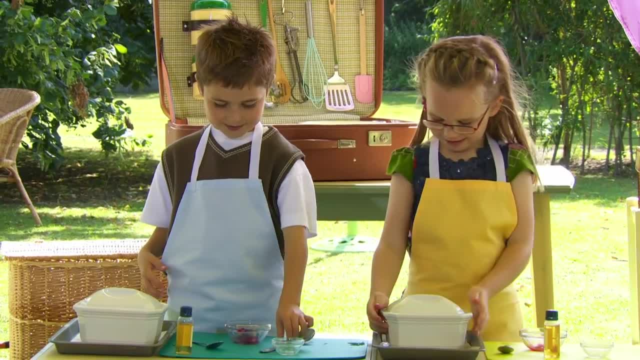 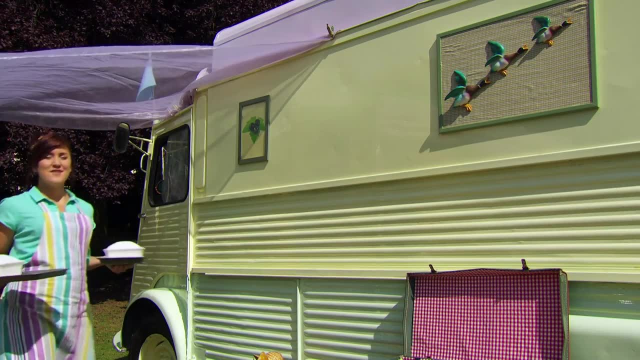 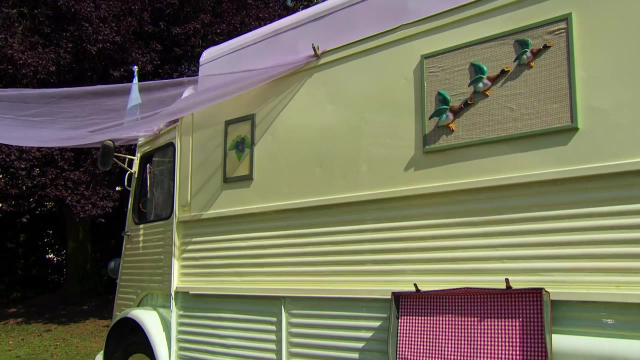 together for your baked black currant rice, and you did it all by yourself. Well done. And now let's put them in the oven. Remember, ovens are hot, so don't go near. Ask a grown-up to help you here. 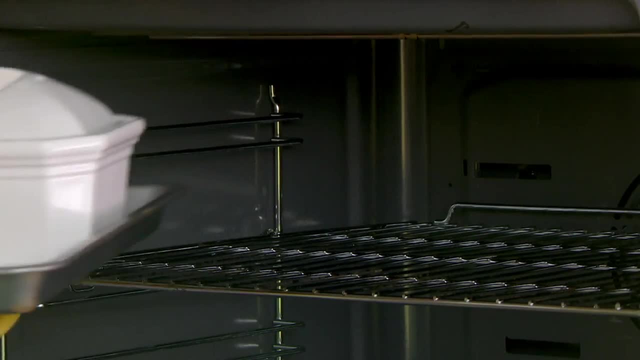 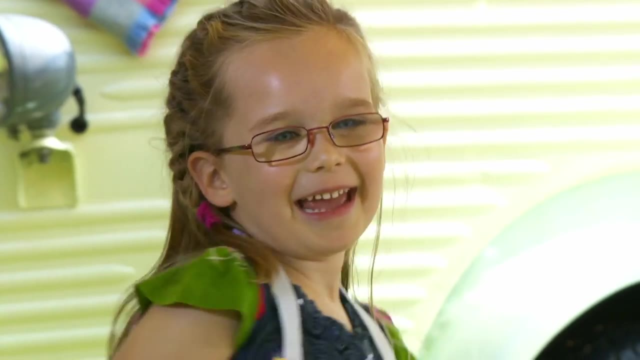 Now. we've cooked with you And had a good time. We've had lots of fun. Let's tidy up and think of all the things that we have done. There was Measuring, Pouring, Sprinkling, Stirring.